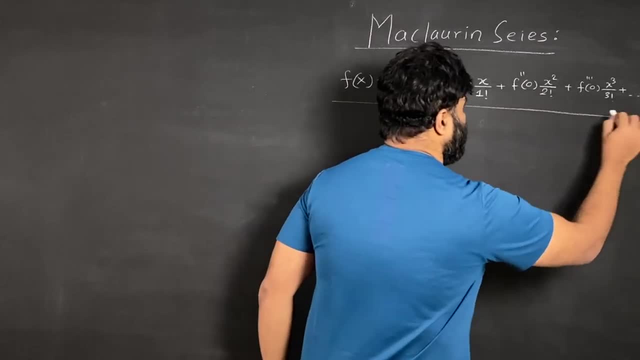 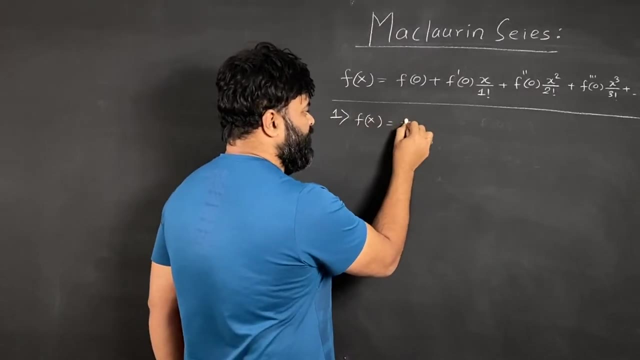 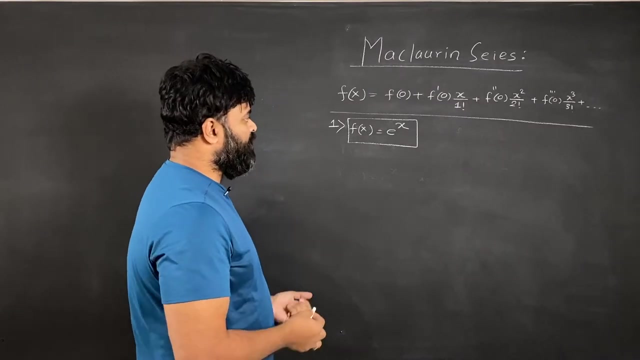 and find the power series of a function. So I'm going to take my first example. The first function that I want to write Maclaurin series for is f of x, is say, e raised to x. Now this is the function we have and we want to find its power series. So let's start Now. I want f: 0. 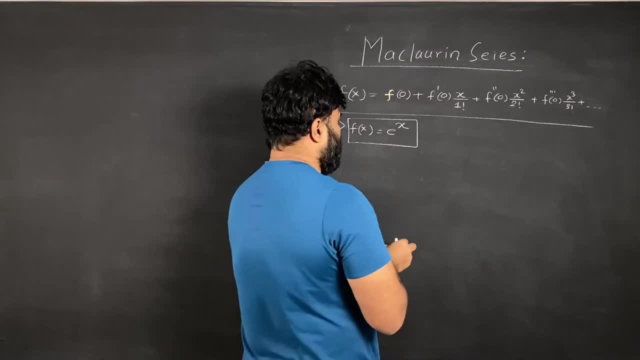 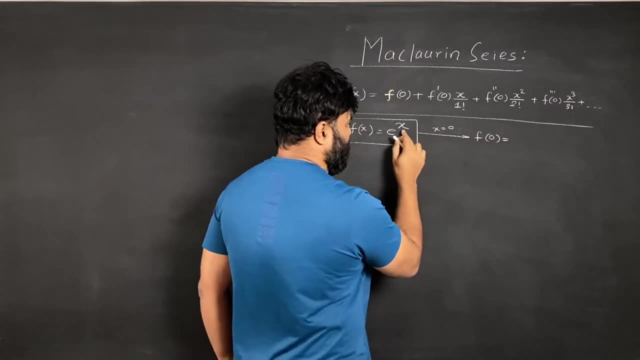 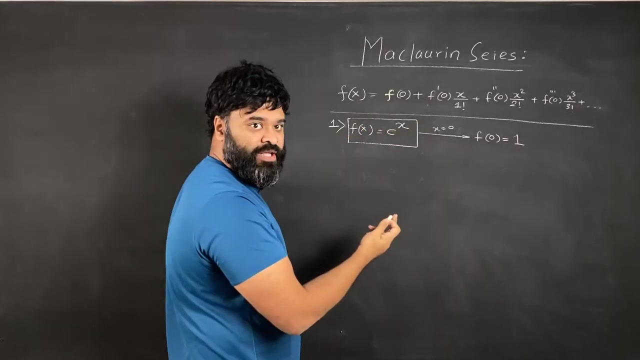 and to get f 0, what I will do is I'll put x is equal to 0 in here. This will become f of 0, and when you put x is 0, it is e raised to 0, which is 1.. Now, next I would like to find: is f dash of 0. 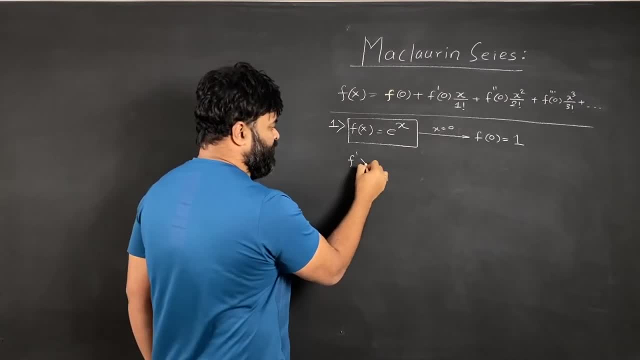 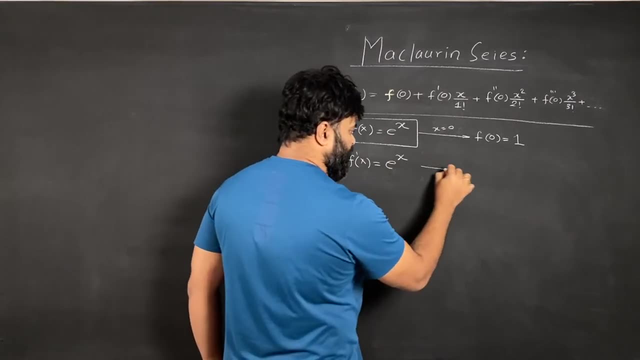 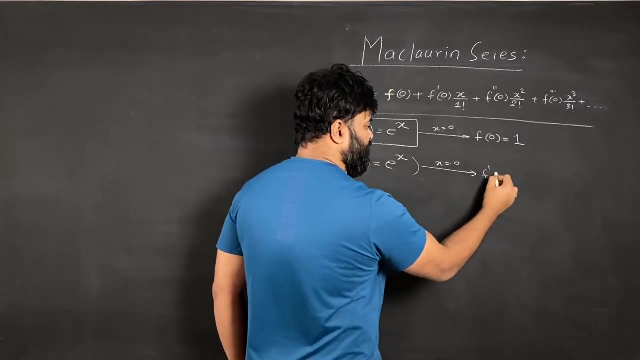 So first I'll have to differentiate this function and derivative of f of x is f dash of x, but derivative of e raised to x is just e raised to x. So I'll write that. and now here I'll put: x is equal to 0 in this. So I'll get f dash of 0 because I put x equal to 0, f dash of 0, and well, that is also 1, right e raised to 0 is: going to be f dash of 0.. So I'll put: x is equal to 0, and well, that is also 1,. right e, raised to 0, is going to be f dash of 0.. So I'll put: x is equal to 0, and well, that is also 1, right e, raised to 0, is going to be f dash of 0. 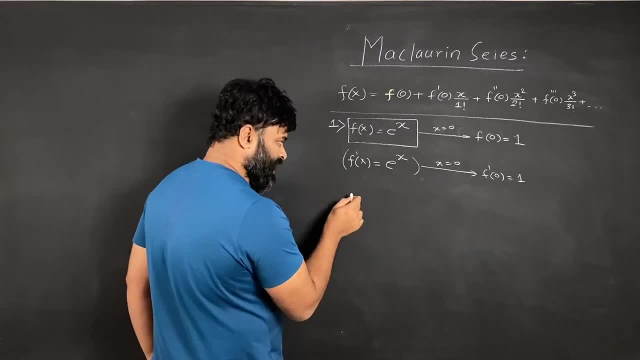 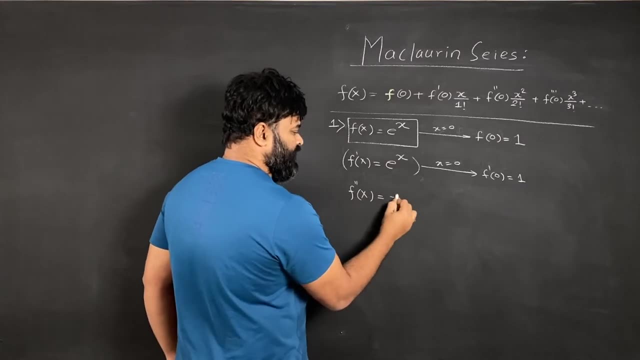 Now, obviously you can keep on doing this. differentiate this again. Now, that is f double dash. That's the second derivative of the original function, f double dash of x. and derivative of e raised to x is still e raised to x. It's a simple example. we're just starting off and we will see. look at some more complicated ones. 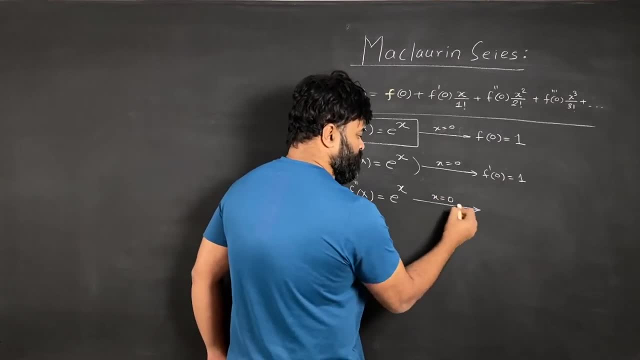 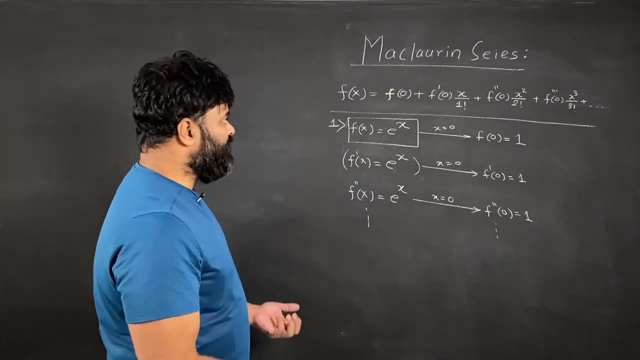 later on. Now, in this also, you put: x is equal to 0, then f, double dash of 0, is also 1, and on and on. you can keep on doing this. Now, what I will do is I'll use this Maclaurin series expression: 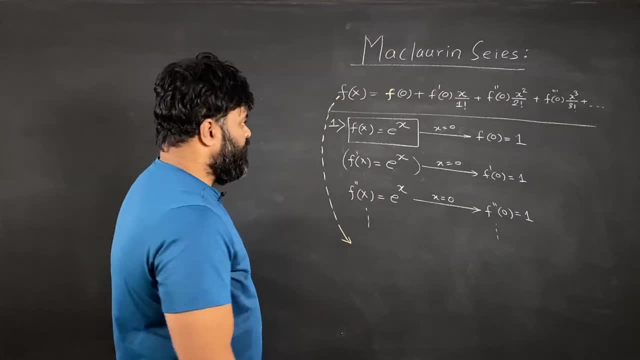 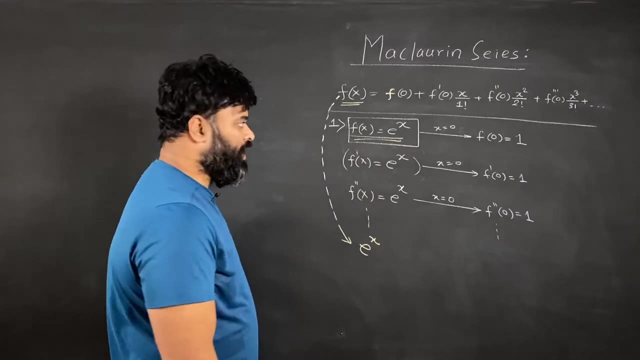 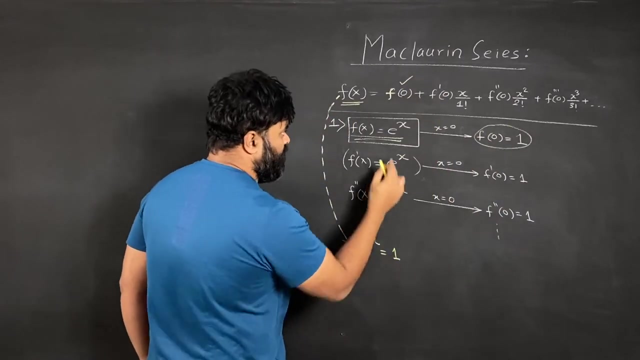 and find out the power series. The f of x is e raised to x, so I'll replace that as e raised to x. I already have f of 0 value, which goes here, and f of 0 is 1.. So the first term, I got this one as 1. 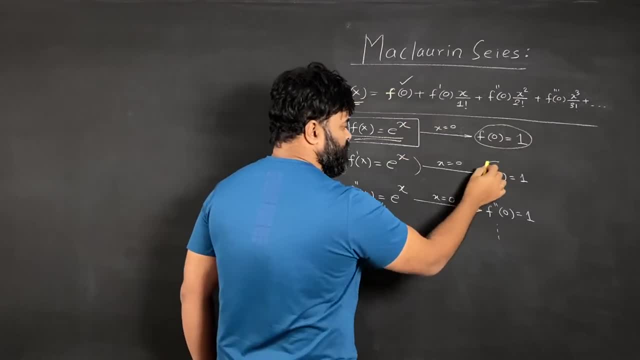 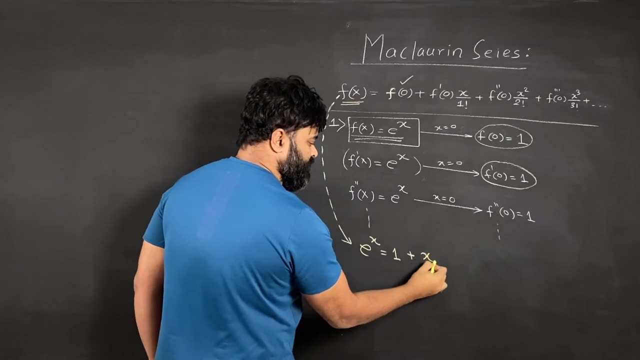 plus f dash of 0 is here, that is also 1.. So when I put 1 here, this will be x upon 1 factorial, that is also 1.. So I'll get x here, So I'll put x here. 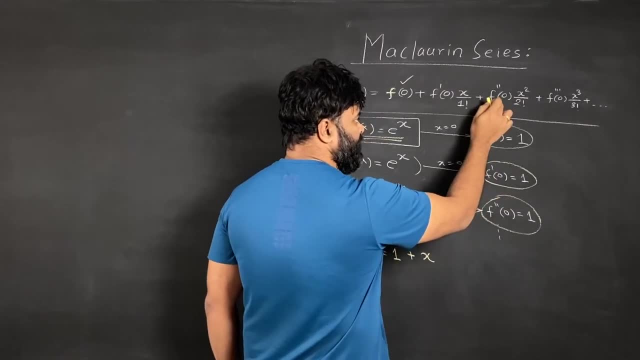 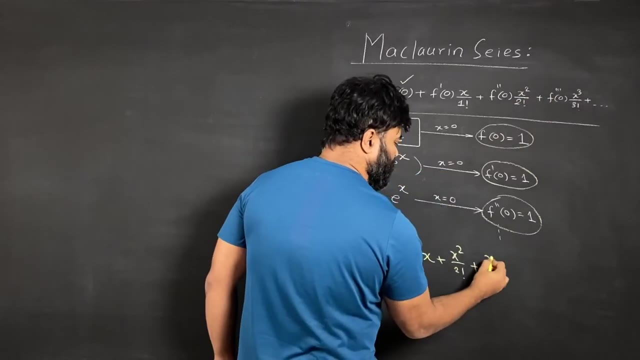 So I'll get x here. So I'll put x here, put f double dash of 0 here, and then that is 1. so I'll get x square by 2 factorial and if I put the third value also, it will be x cubed by 3 factorial. 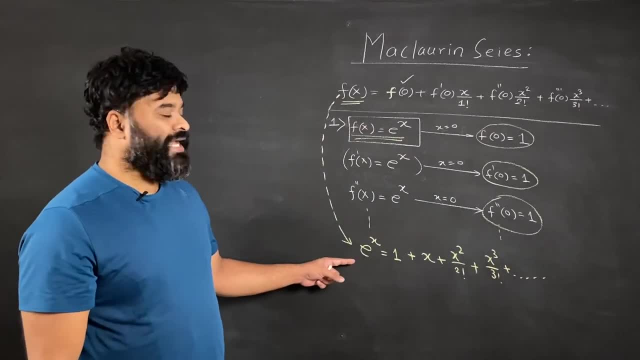 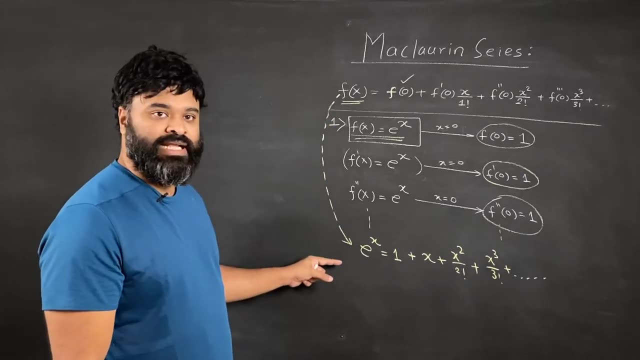 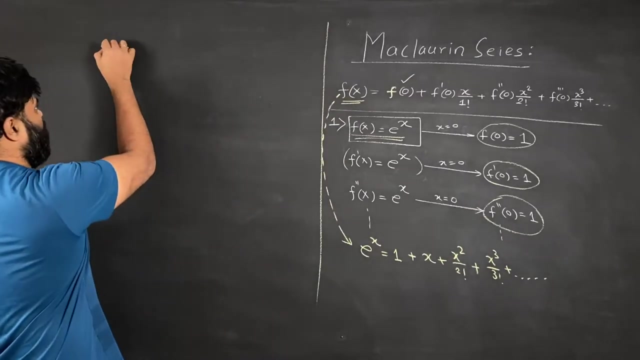 and so on, and what I obtained here is a power series of erase twigs- a very simple example- and I showed you how you use this power series, the Maclaurin series, to find a power series. now let's go to slightly complicated example now. second function that I want to talk about is: let's say, f of X is equal to: 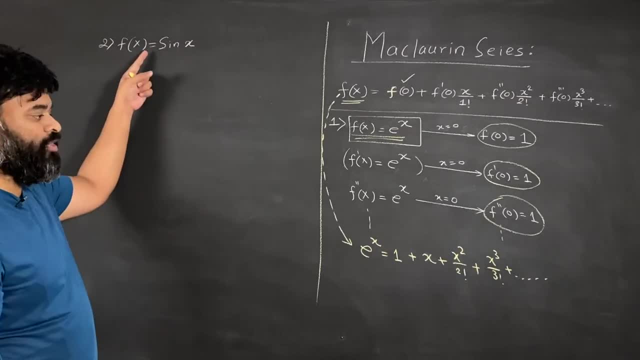 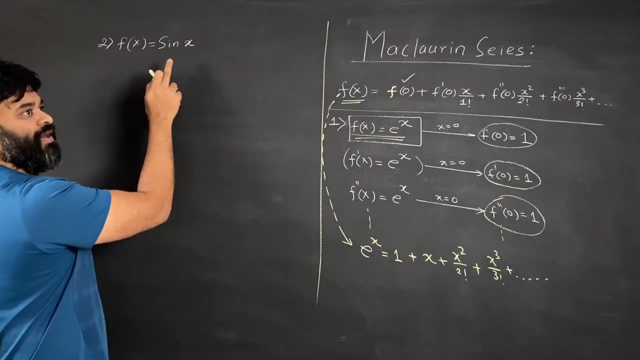 sine X. now for sine X, we want to find power series, like we did for erase twigs, and let us see how we can do that. now. procedure is pretty much same for every function and its derivative. you put X equal to 0. so let's say I put X is equal. 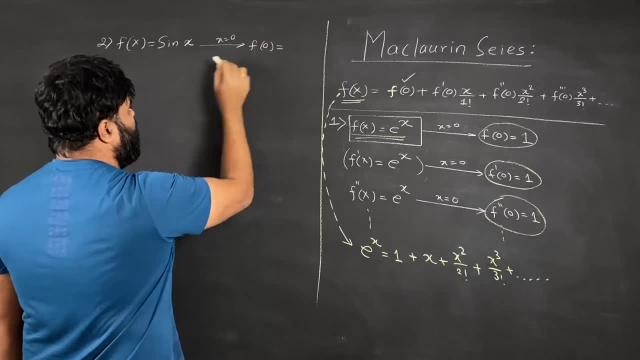 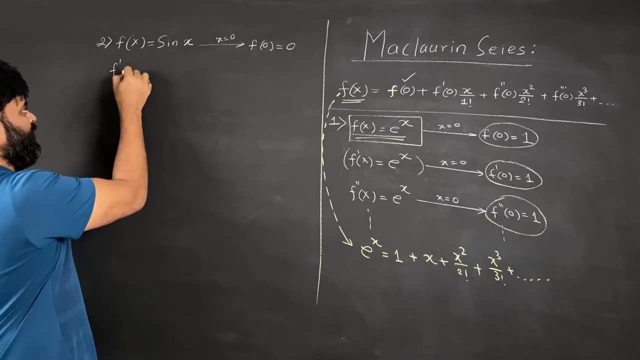 to 0. to this I'll get f of 0. and when I put 0 here, sine 0 is 1, sine 0 is 0, right, so f of 0 is 0 in this case. now keep differentiating, right. so I'll put f of 0 here. sine 0 is 1, sine 0 is 0, right, so f of 0 is 0 in this case. now keep differentiating. and. 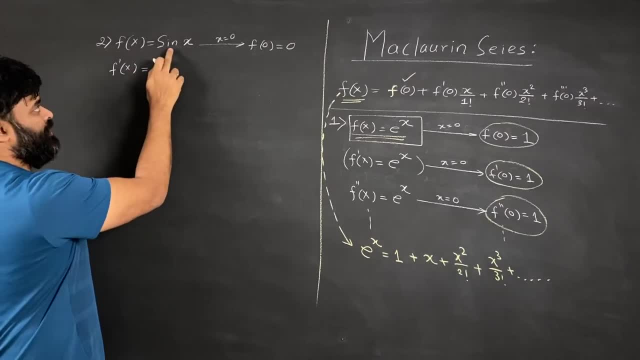 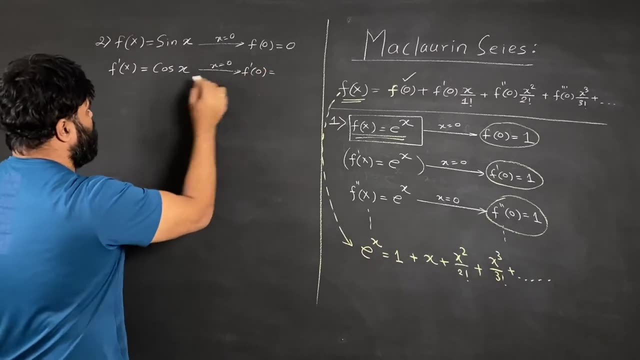 f dash of x. the derivative of f of x is f dash of x. derivative of sine X is cos x, and then put x is equal to 0 to that, so it is f dash of 0 and cos 0 is going to be 1. so this: 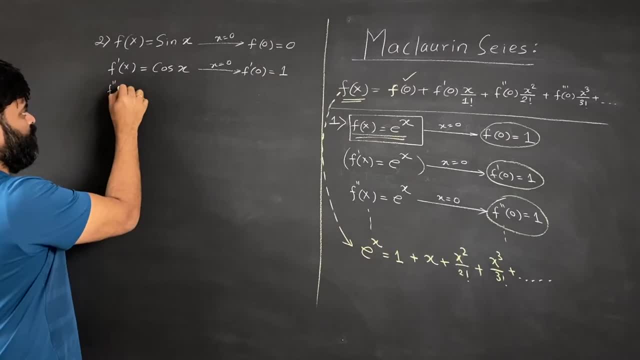 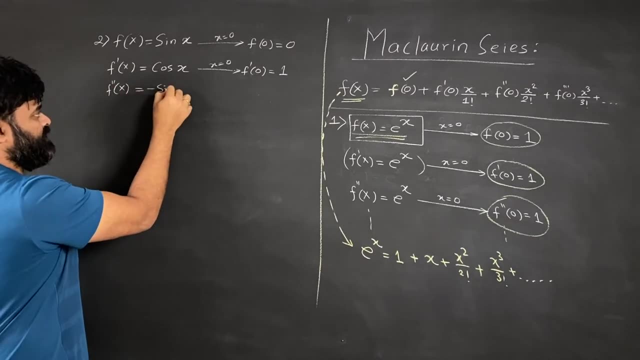 value is 1. now differentiate again. let us do that some more. f double dash of x, that's the second derivative of the original function. derivative of cos X will be minus sine X, so negative sine X. and now you put X equal to 0, sine of 0 is anyway 0. 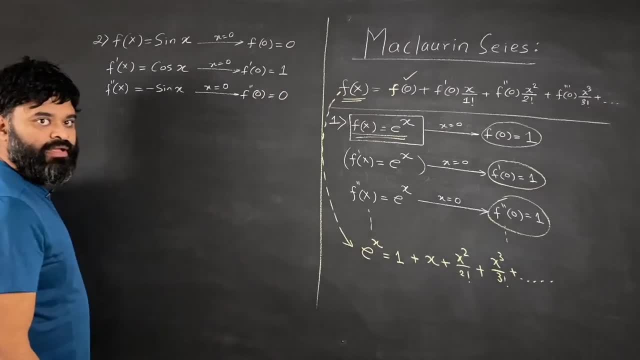 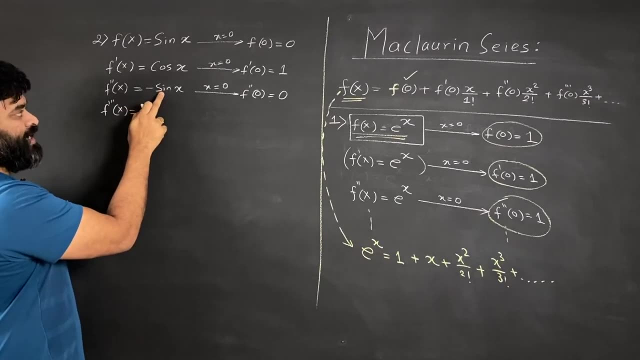 So f double dash of 0. also, we got 0. Now let's do some more. we will need those terms. So let's say f triple dash of x. the third derivative, third time derivative, Now derivative of sin x, will become cos x and this minus sign will carry on. 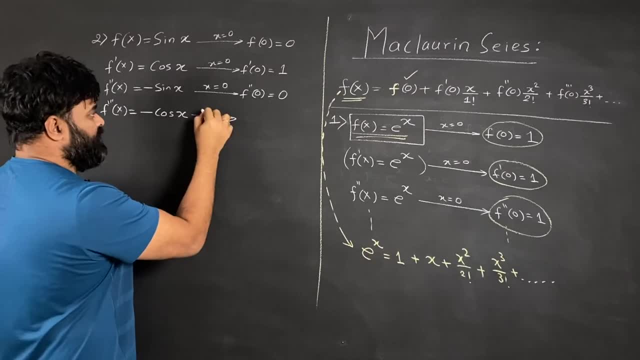 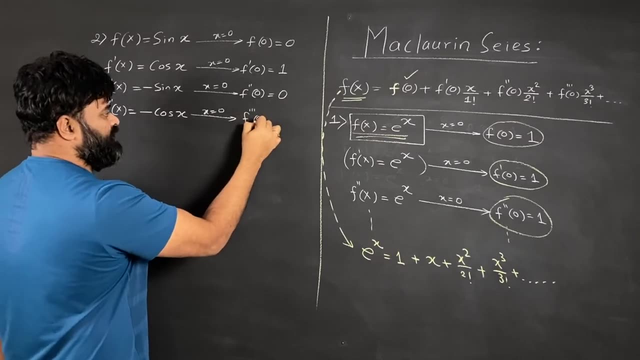 So it is negative cos x. And now you put x is equal to 0, this will become cos 0, okay, And cos 0 is 1, so you get negative 1.. So f triple dash of 0 is negative 1.. 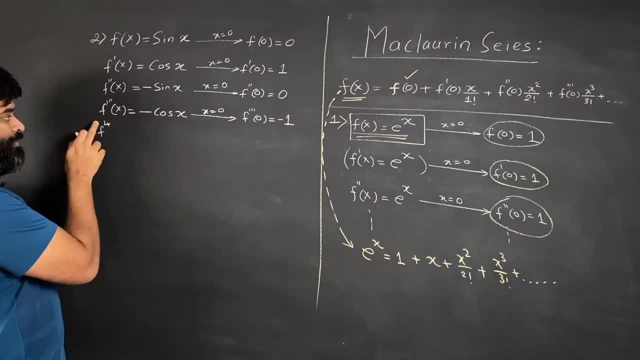 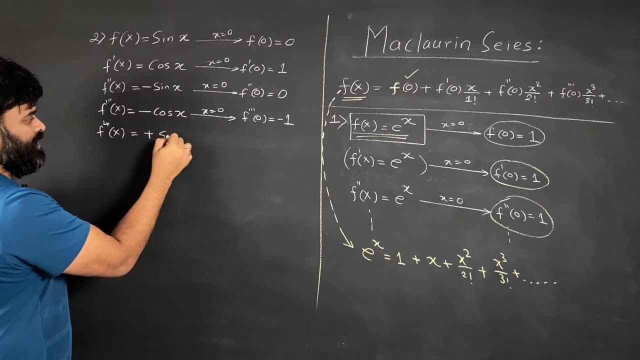 I want to do a few more And you get it right. The fourth derivative- I might want to write f4 of x, That is, derivative of cos x will be negative. sin x will make it plus sin x. Just be careful with the sign. 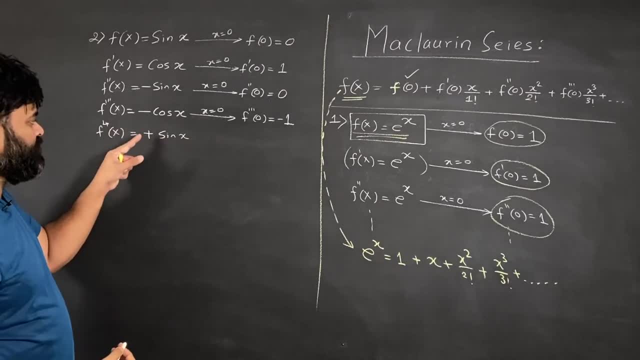 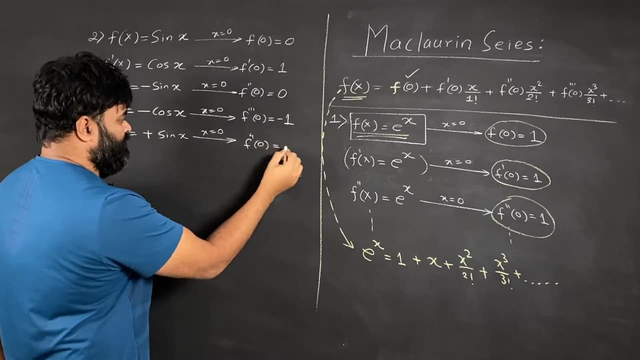 The derivative of cos x is minus sin x and because there is minus sign outside, this will become plus And I will get this as now. I will put x equal to 0 again. This is f4 of 0, the fourth derivative. 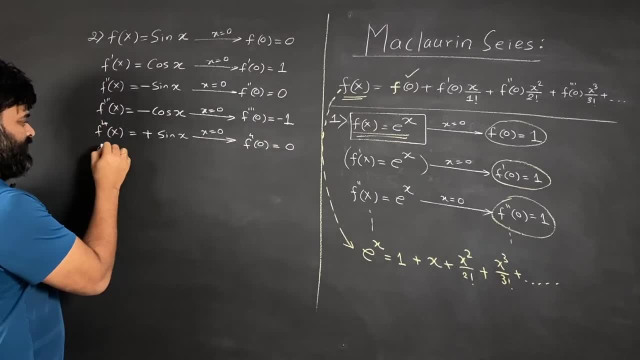 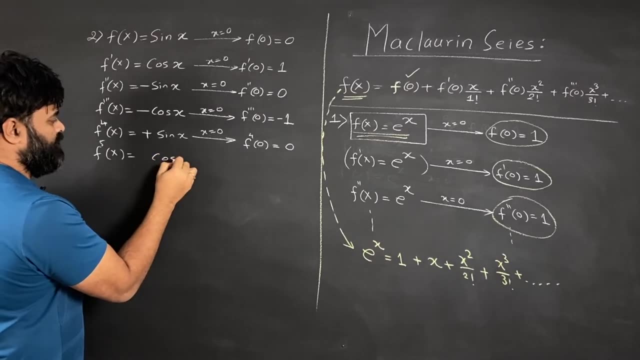 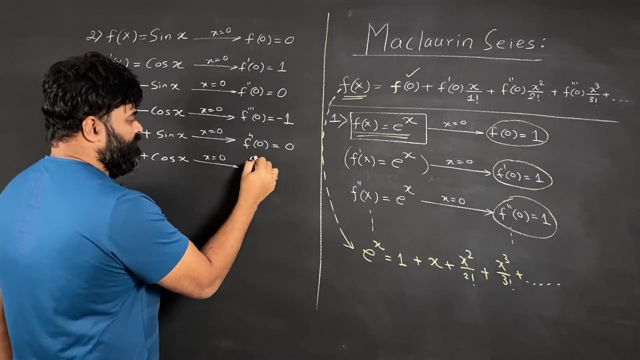 Well, that's 0 again, no problem. And one last. that's it. So fifth derivative of x, f of x, is going to be derivative of sin x. This is going to be cos x, and this time it is positive. and then you put x is equal to 0 to it, it becomes f. fifth derivative is 0, and I plug in x 0 here. this is cos 0, cos 0 is 1, okay. 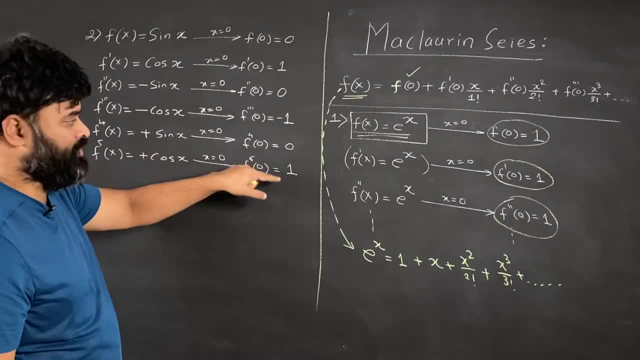 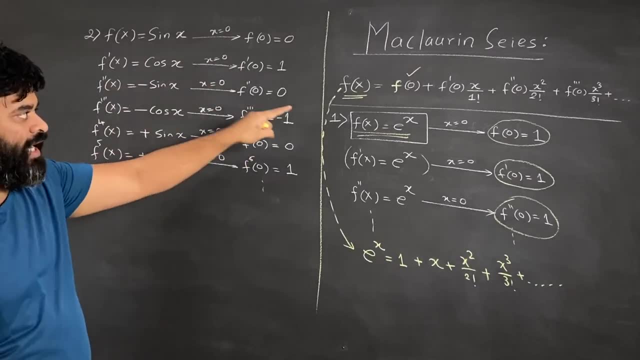 And then you see there is an alternate: plus 1, then 0,, then minus 1.. There is a pattern to it. of course, it's a series, right? You can keep on doing this Now with all these values. I'm going to use these values and the MacLennan series to write down the series, the power series. 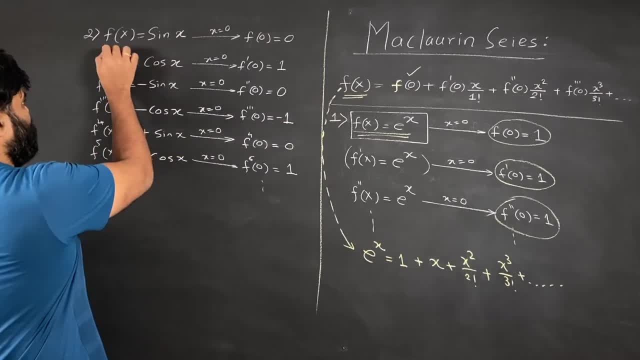 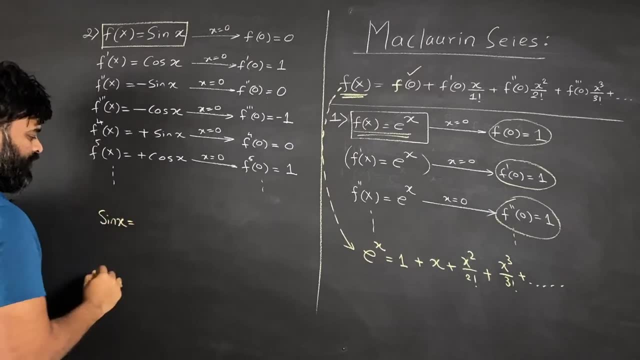 Okay, These are sin x. Now the function this time is sin x, right? So I will put that here. sin x is equal to- I'm going to write down all the terms nicely. We have f of 0,- this time it's 0, which I will go here. 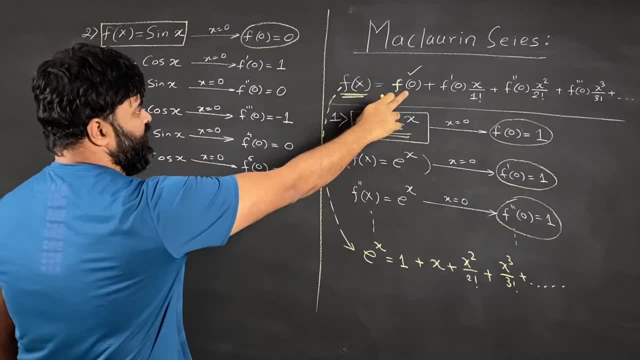 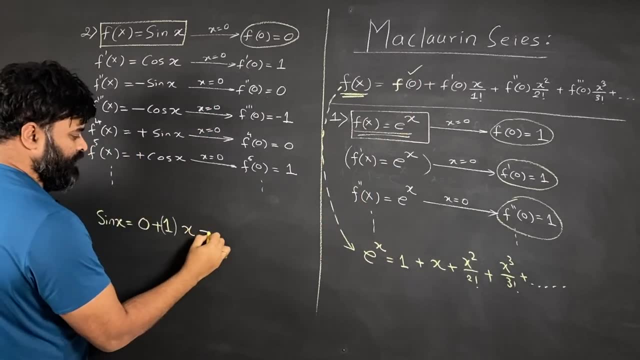 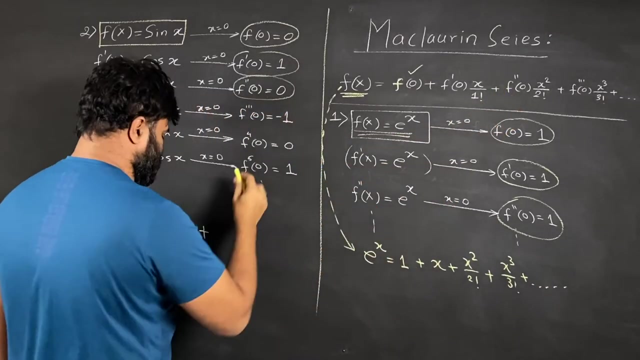 I write 0 plus now. next is f dash of 0, which is 1.. This value is 1 here, and it is x plus okay, f dash of 0, done. Now I will put f Double dash of 0, that goes here, and then that is 0. 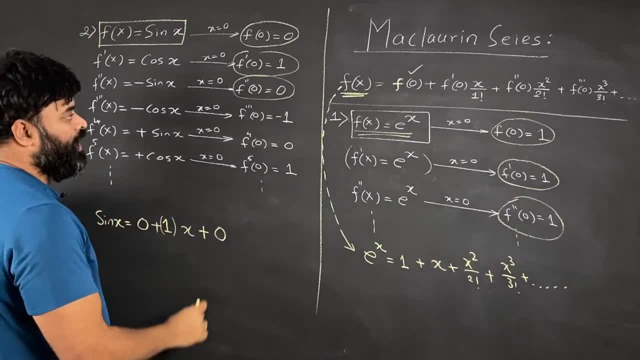 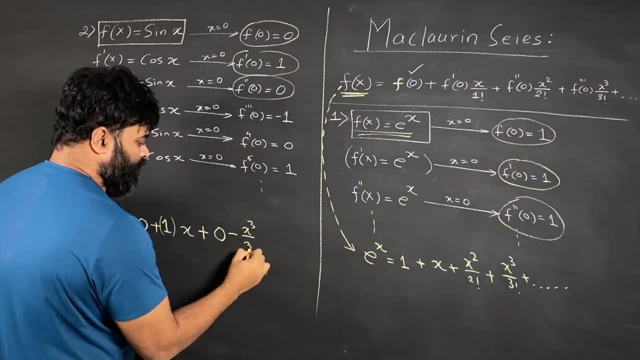 So the next term is 0. You see, alternate terms are working out to be 0. Then when I put f triple dash of 0, which is minus 1, that goes here. So it is minus of x cube upon 3 factorial okay. 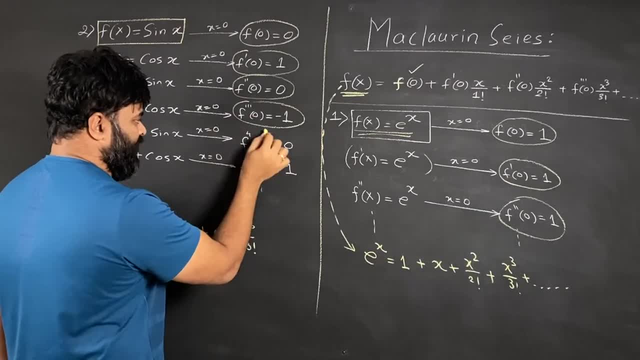 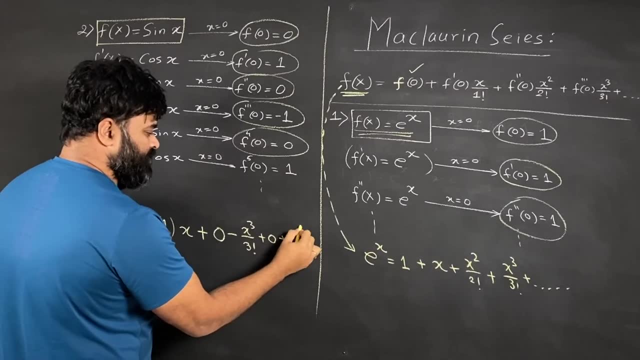 I hope you can imagine the next. this is f triple dash done. f fourth derivative is going to be 0 and f fifth derivative is plus 1.. So it is plus 1 x to the power 5 over 5 factorial. So that way I got the sin x power series. 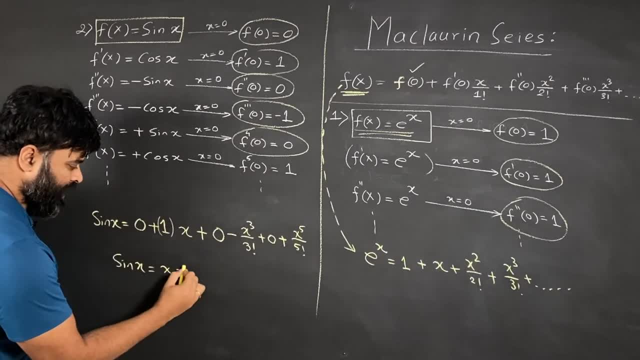 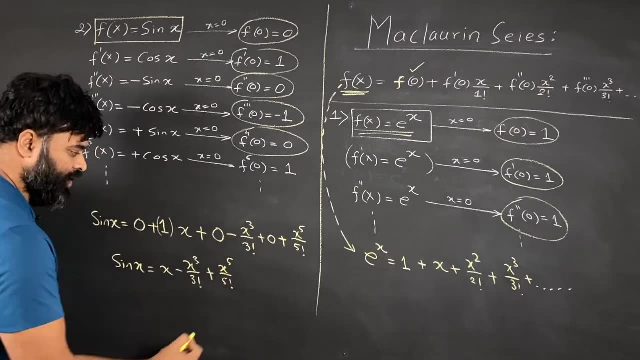 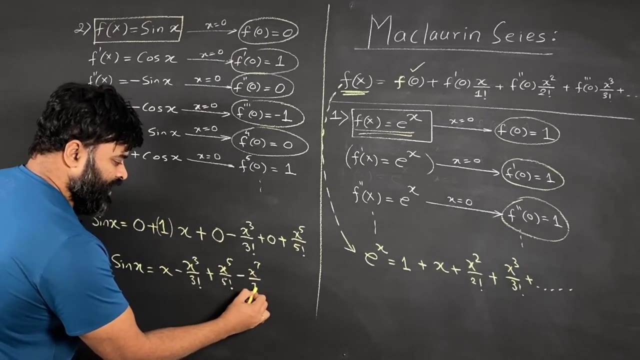 The first term I write is x. this is anyway 0, minus x cube upon 3 factorial plus x to the 5 divided by 5 factorial. And when we say series, you can always predict the next number. And the next number is going to be x to the power 7 divided by 7 factorial, and so on.